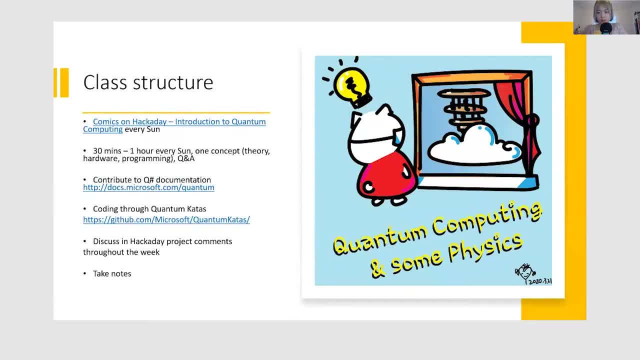 Thanks, Nathan, for posting the link there, and if people can also mute themselves, that would be helpful. Thanks, The materials that we use in the class. we refer to the Microsoft Q-Sharp documentation and we also use the quantum katas for exercises. 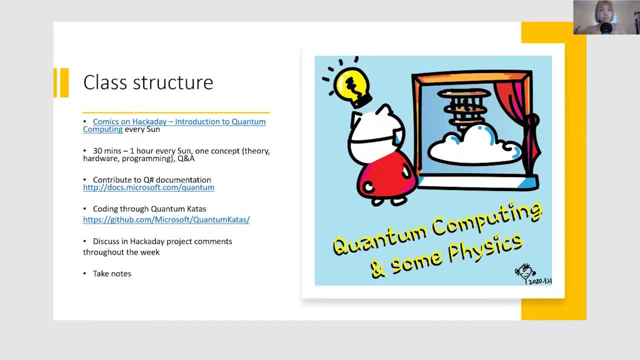 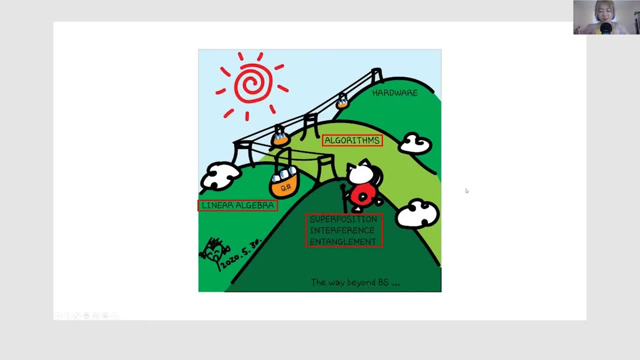 So today we're going to also do a katas. Actually, a kata is singular, So people have seen almost every class. now that we have this landscape that tells us where we are and what we're doing for the class, and we use the Q-Sharp as a way to 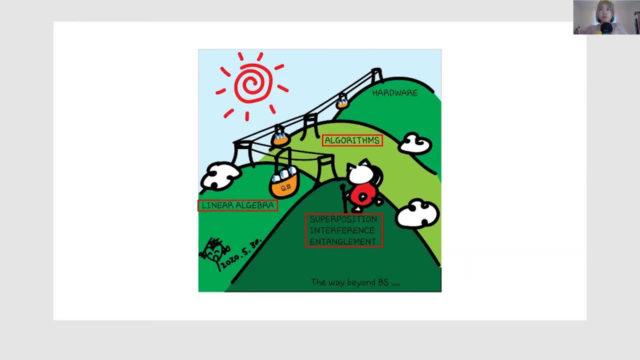 connect from the concept to coding algorithms. So previously we have done quite a few algorithms that's based on superposition and in entanglement, like teleportation, superdense coding. Those are using entanglement for interesting communication purposes. There are a lot of other algorithms that are using all of these properties. 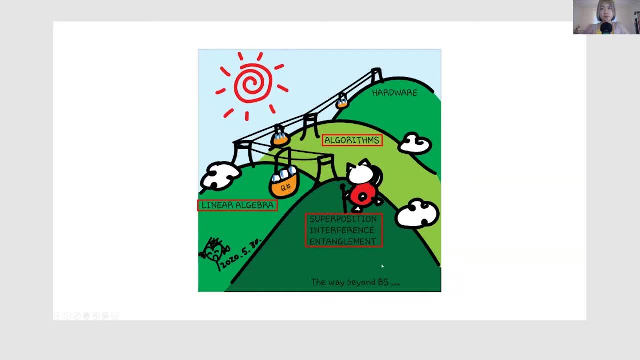 So if we put entanglement and interference into the same algorithm and use all of these behaviors from quantum computing effects, that can be very interesting and powerful. So today we are going to look into a particular algorithm called Groover's algorithm. 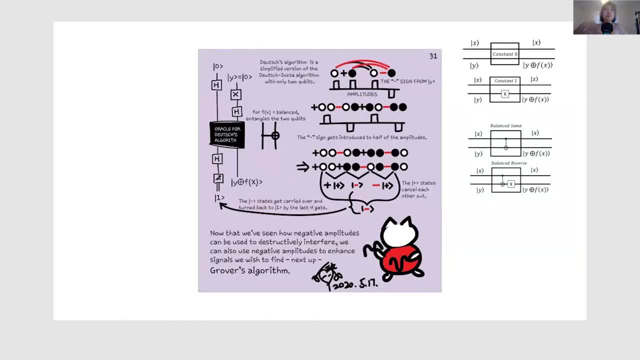 Before that I have this reminder here: We have seen in some previous classes the Deutsch algorithm and Deutsch-Hauser algorithm, where we did look at a case where entanglement- sorry, interference- was very important. So namely when you can have interference happening when you introduce a negative sign. 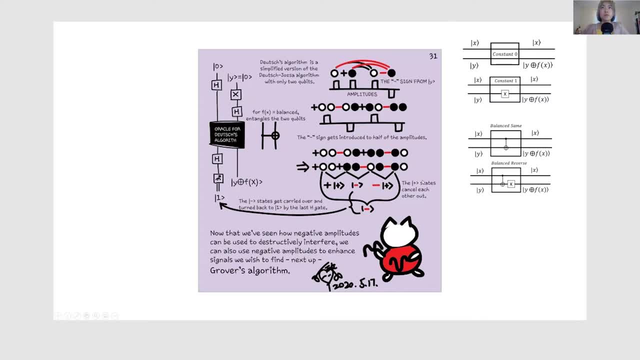 you can distractively interfere with some other states and reducing the probability of that state being in your measurement result. So this is really useful. if you use this interference behavior in your set up, you can extract information efficiently. So this is Deutsch's algorithm. 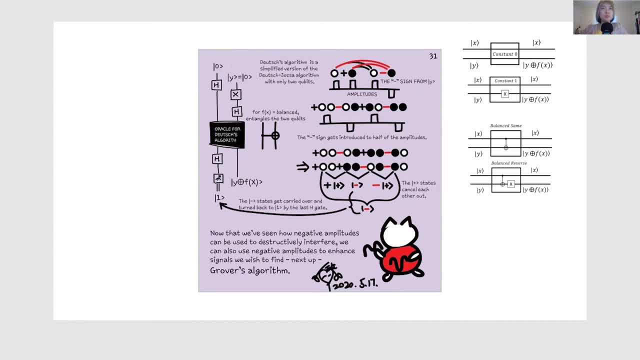 We're not going to do. I don't think we need to do another coding exercise, although there are quite a few on the quantum kata. So if you are interested- and I definitely encourage you to go to the kata and try the Deutsch algorithm and Deutsch-Hauser algorithm using the kata. 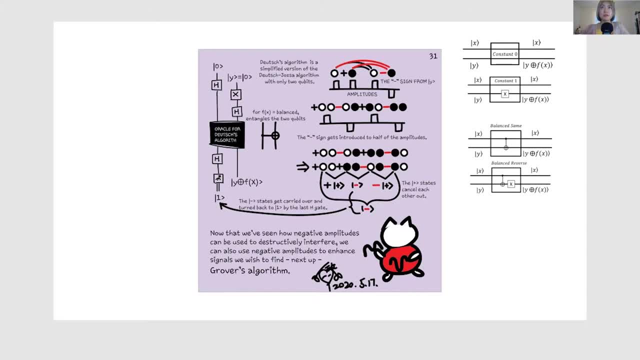 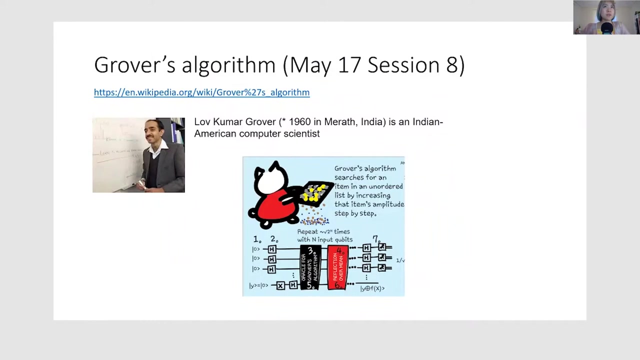 And if you missed the conceptual class about this, we have that in the previous list of classes. you can watch the recording for. But we're going to use today's class on Groover's algorithm because that's a useful algorithm. It's also one of the most famous algorithms that was invented or came up with. 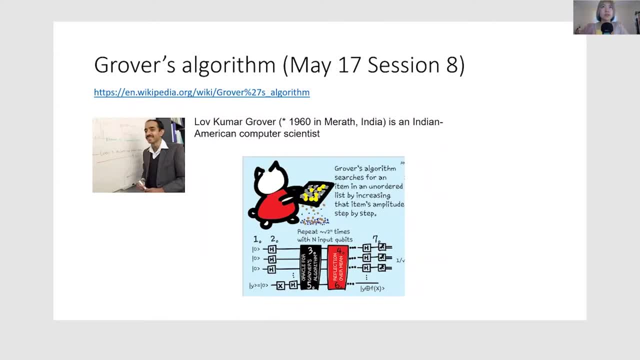 by the Indian American computer scientist Groover And we did spend session eight on discussing the topic and concept about this. but we would do a revision today And if you want to see the previous one, go to the May 17th session. 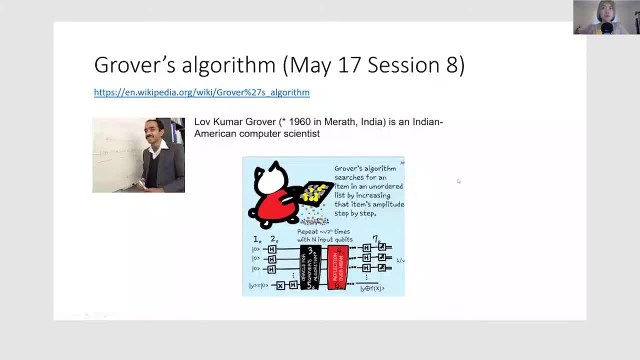 This one, as well as the Schwarz algorithm, are the ones that you can actually use for some applications, Whereas Deutsch's algorithm and Deutsch-Hauser are more academic algorithm that were invented early on in the development of quantum computing, So they do not have real use cases. 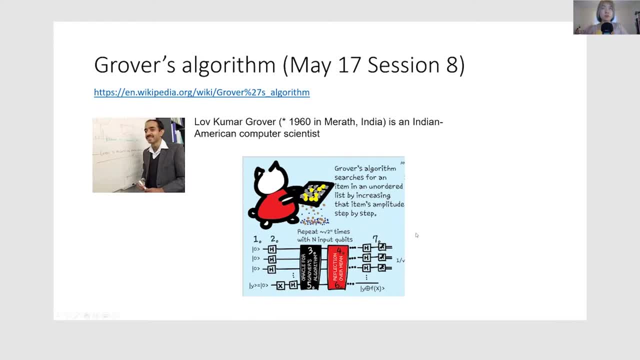 but they are very useful in terms of learning and understanding. We can also use Groover to gain some intuition and understanding of using superposition interference entanglement in the algorithm setup. So, broadly speaking, if we just zoom out, not looking at the details, 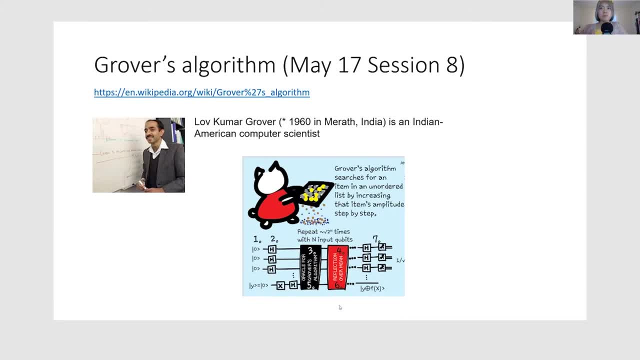 what this algorithm does is trying to search for an item in an unordered, un-sorted list, and it's like doing this selection here. It can increase the amplitude or probability of the item that we're looking for, And it's consisted of a couple of boxes that we need to run in iterations. 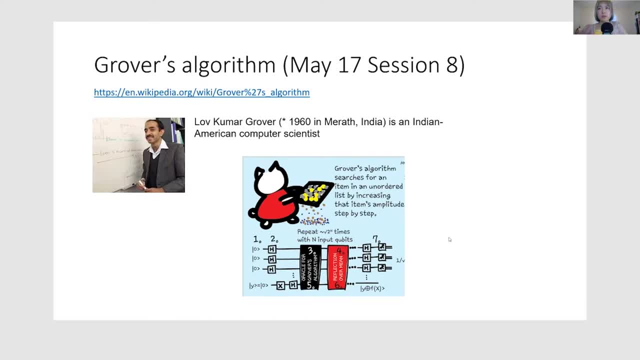 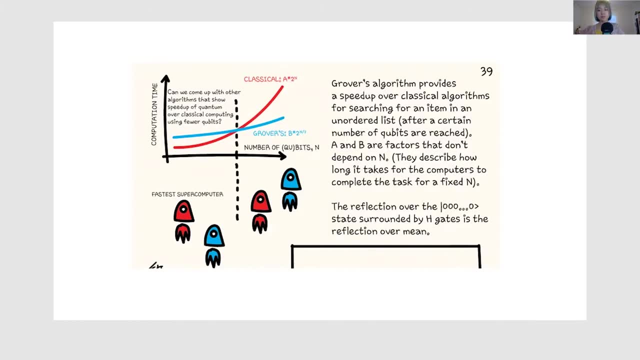 The Groover's algorithm. you can use it for searching an item, And you can do that. you can do that using classical algorithm as well, And classically, if you want to search an item in the list, then you may have to. 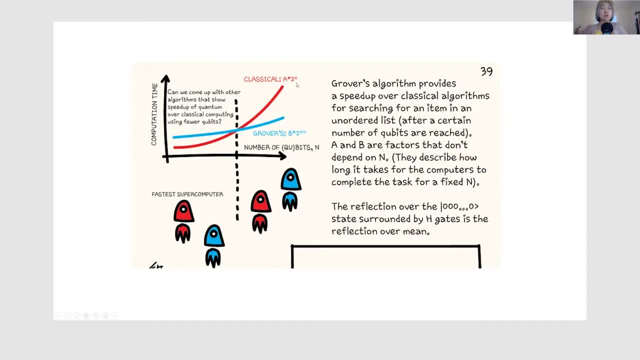 if you have n bits you may have to run your algorithm up scaling with two to the n. But for Groover the scaling is two to the n over two, so square root of two to the n. Then at first, if you have a small number of bits, 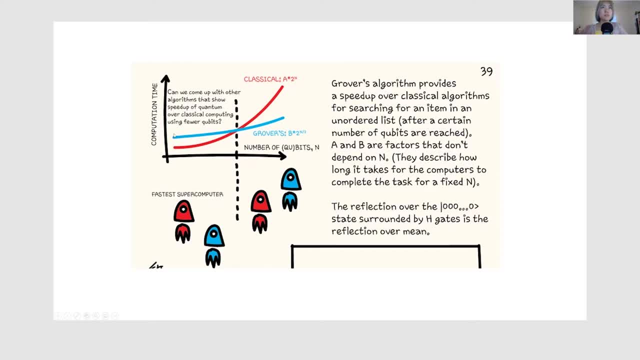 it may not be a speed up. So this is something that we have to keep in mind: that this algorithm would be advantageous once we reach certain qubit numbers. So it's like this race between a supercomputer and a quantum computer. where at this region? so maybe a small number of qubits. you can just do it with a classical computer. There's not much reason why you would use a quantum computer to run it. But when the number of qubits gets really large, then that's when this Groover's algorithm really can take off. 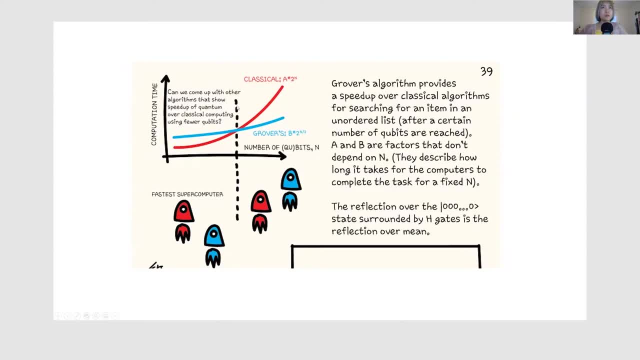 So we don't quite know the exact number that's needed. So let's look at the curve. You see that the graph is a little bit different. It depends on the number of qubits, depending on where this will occur. It depends on a couple of things. 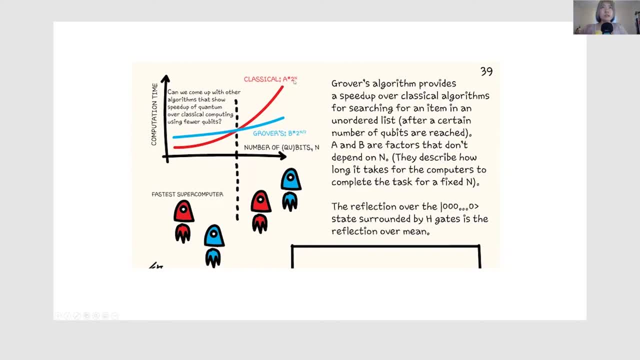 So the classical versus quantum, these scaling, these are the scaling factors, but we don't exactly know the factors for the supercomputer or quantum computer because we don't know exactly how many qubits are needed, quite know what would be the best kind of 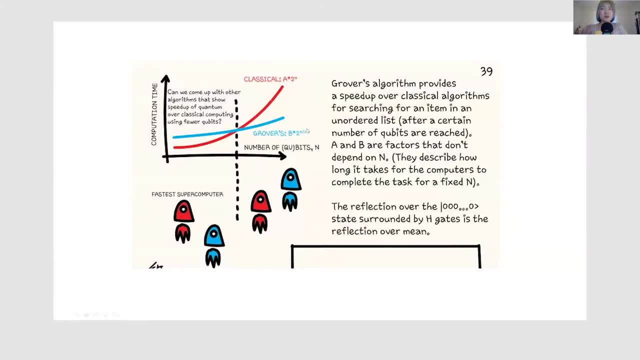 supercomputer and the best quantum computer. yet Of course we're still building quantum computers and there are so many different types of architecture. So this: how much running one of the algorithm, running it once, would take, we don't exactly know. We don't exactly know how many numbers of. 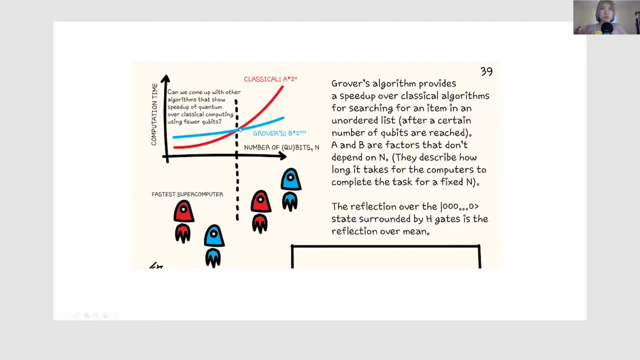 qubits that we will need to see this crossover, But then we know that it's going to be a large number. Then if we look at smaller numbers, we have to come up with a lot more algorithms to really show at the low number. 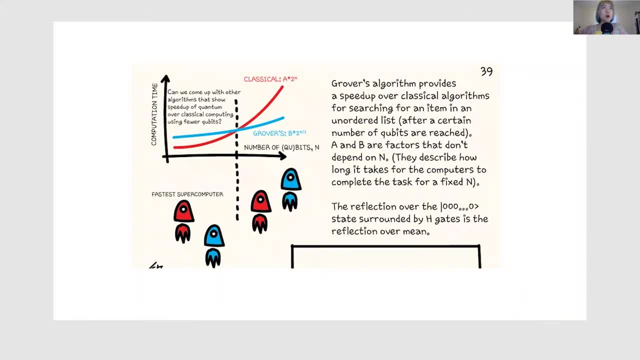 can we come up with some useful, interesting algorithms that could have quantum computers be more advantageous. So this is definitely all of these are both the hardware and the algorithms- are depending on all of us when we are doing quantum computing development, both in terms of software and 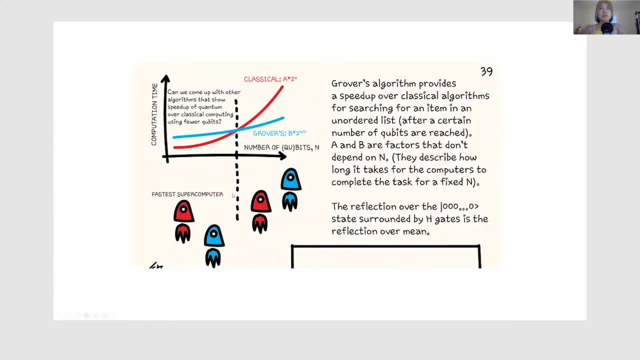 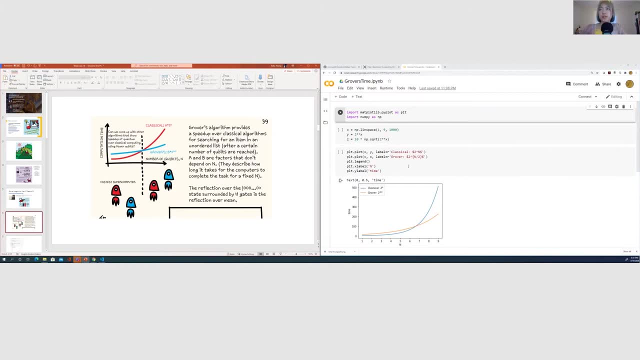 algorithm development as well as the hardware. I did also make a little plot just to show this concept here. It's not that, of course. if we look at the scaling factor, Groover is square root of two to the n, classical is two to the n. 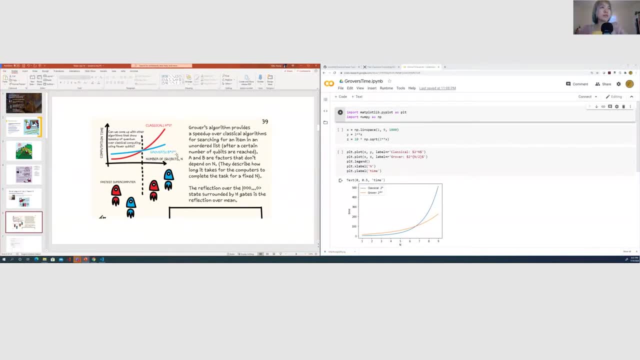 and it seems that Groover will be faster. but then we don't know what the prefactors are. So if you want to see how this scaling goes and you can put just fictitious factors in front of them, that in this case I'm putting, b equals to 10 and a equals to one. 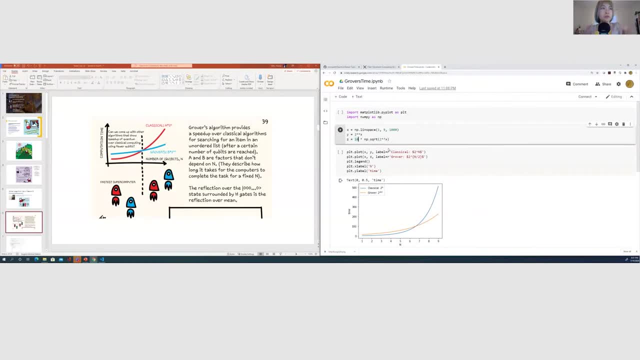 That's just a fictitious guess, because that really depends on how good your hardware is and how fast, intrinsically, your computer will run one iteration of your algorithm. So yeah, just some additional emphasis that I didn't mention in the last class and also some food for thought there. 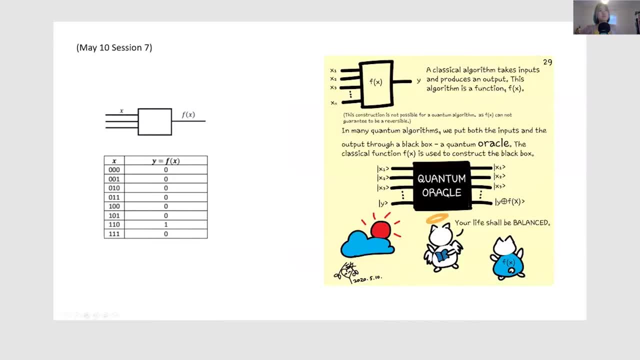 Okay, So when we are building a algorithm, we will need to have this oracle. When you want to use interference in your algorithm, this oracle is like a black box. We have learned about this in session seven on May 10th and we use the Deutch-Holzer algorithm. 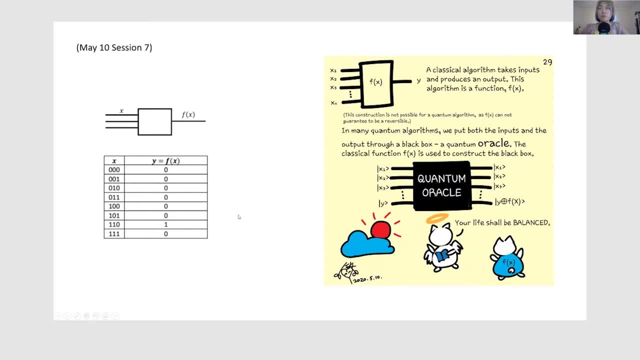 to understand concept of quantum oracle. So for people who have missed that, definitely go to that session. We won't be repeating that. So, in short, when we are building a quantum algorithm, we need these oracles that functions like inputs of another part of the algorithm. 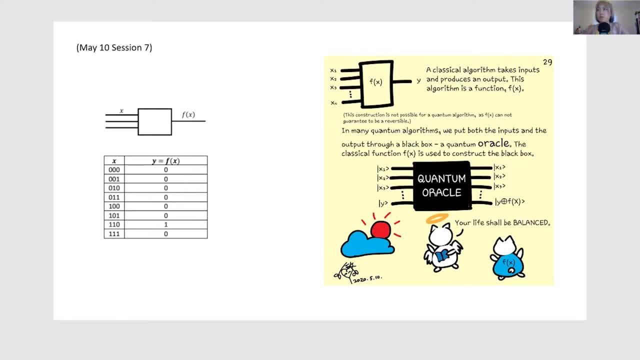 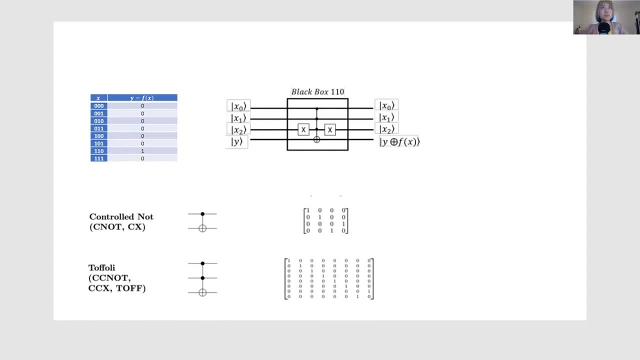 And for a groover we can build several different types of boxes depending on which item we're searching for, For example, the black box for one-on-one. So if we just have three qubits that we are interested in, we can just arbitrarily say: 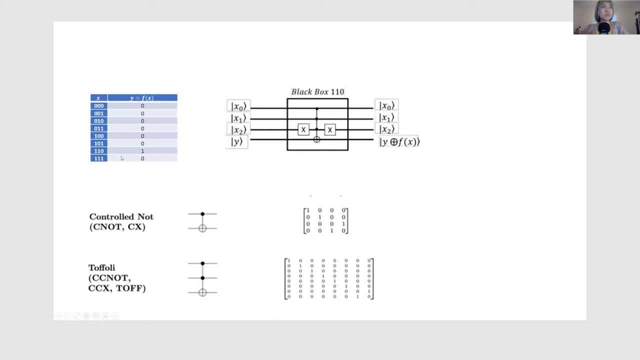 one-one-zero is what we are looking for And the label of that. so Y of f of x, we expect it to be one and the other ones would output zero, In order to build a black box that would pick out one-one-zero. 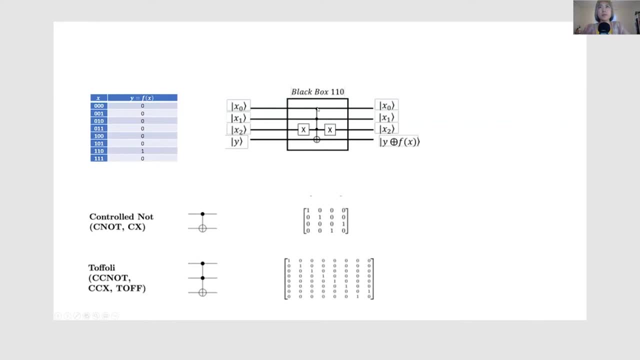 we need to construct this kind of controlled gates. So, if you remember, the control- not gate- just involves two qubits and the first one is the control, the second one is the target. Only when the first one is one, the second one would flip from zero to one or from one to zero. 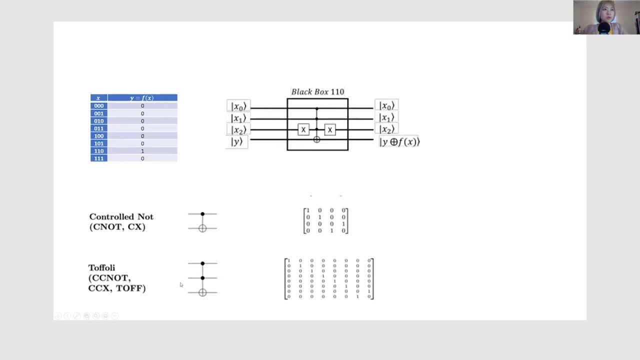 If you have three qubits. this is called a CC knot is also called a Toffoli gate. It has the first two qubits being the control and the last one being the target. Again you have. you can only flip this one when the first two are both zeros. 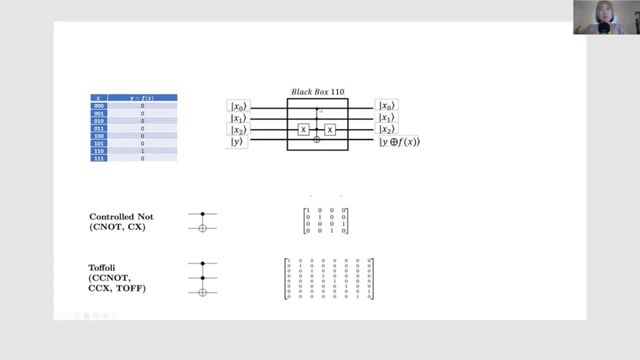 Now you have more qubits. you just add up this control bits. So the requirement of this control gates is that the first all of the other qubits need to be once when your last one can be flipped. So then this means that one-one-zero wouldn't work. 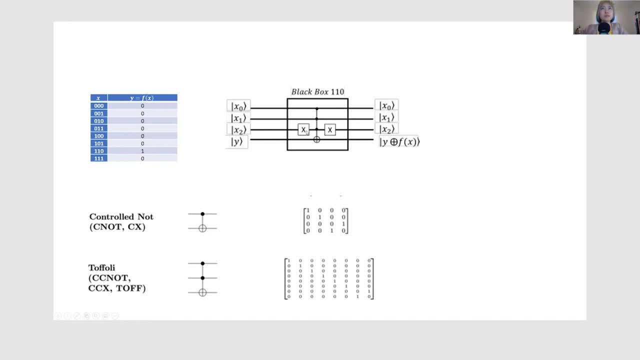 unless you put these flip gates around it- So especially this one, because that would flip from zero to one- then you can change this qubit here. So that's how you set up a black box. I forgot to mention that Oracle also needs to be set up in order to. 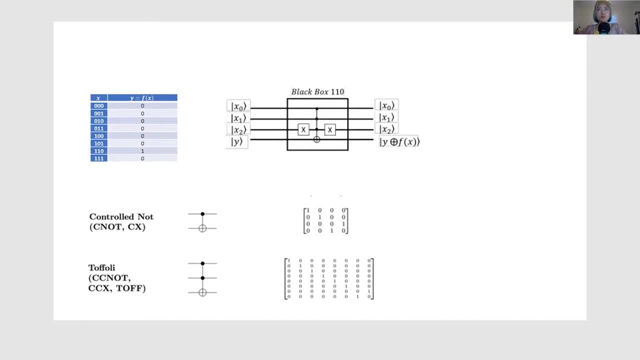 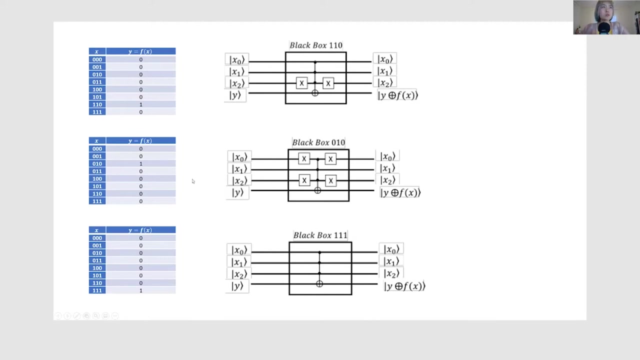 make a unitary operation. So that's another need for setting up Oracles. If these all sounds very new to you, definitely go back to the previous sessions. So similarly, you can build other types of other black boxes, still using three qubits as examples. 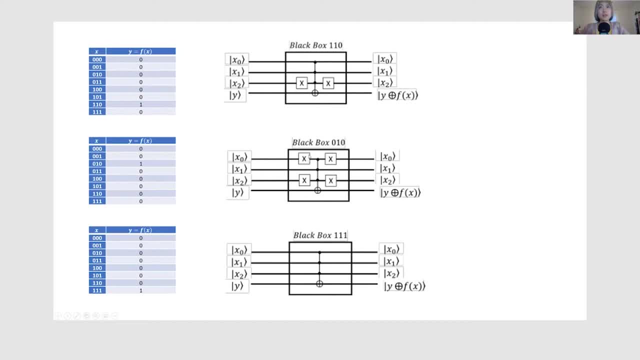 For zero-one-zero, you will have the X gates set up on both the zeros. If you have already the one you want to label that, you don't need to give it a flip, because this already can flip the last qubit. So this is the part that you need to set up first as your Oracle for Groover's algorithm. 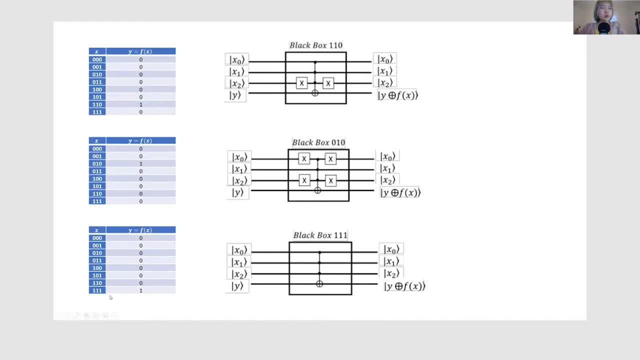 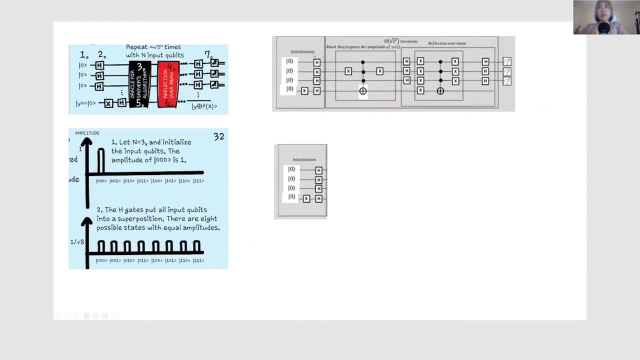 which would then label or mark your item on the list. If you look at the complete diagram for Groover's, again using just three qubits, because that's not too many qubits and not too few qubits, We can still do some calculations by hand if we get lost. 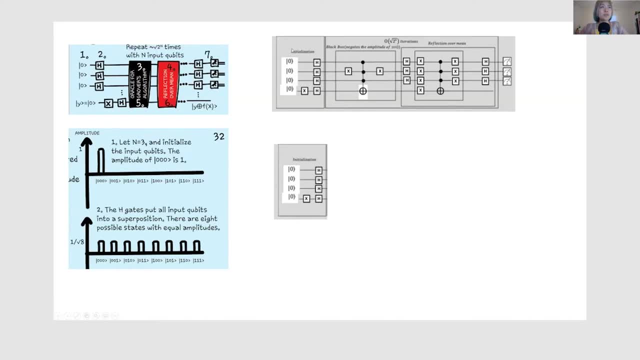 This first part is making everything to equal superposition. When you start with just zeros in your system, you will have this maximum amplitude for zero-zero-zero. The other options are not there, But if you scramble them with the H gates they would make all of your qubits into a superposition of zero and ones. 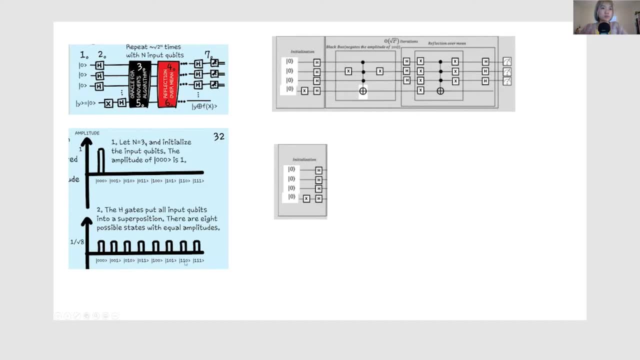 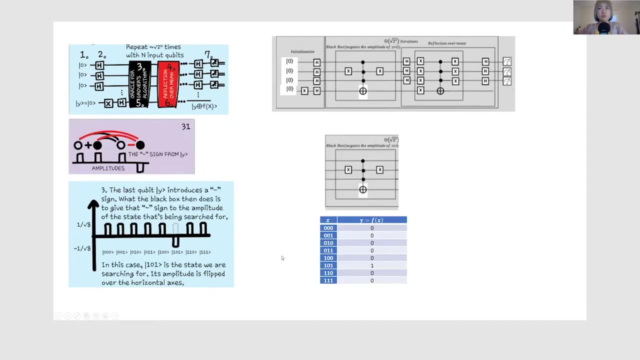 Then you have all of these possibilities in superposition and they all have equal amplitudes. That's what this part does. Then the second part is the black box, the oracles that I've already mentioned introduced. What this does is, if you want to set up a one-zero-one black box, 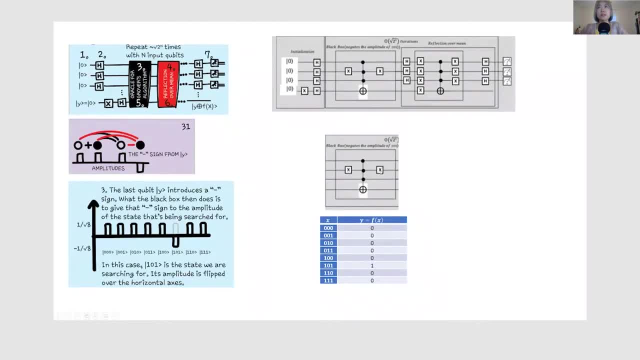 you would put the X gates around your second bit, because your second bit is zero. Then what happens in here is then this very last bit is used to introduce a negative sign. This negative sign would then be scrambled into your whole entanglements or this controlled setup. 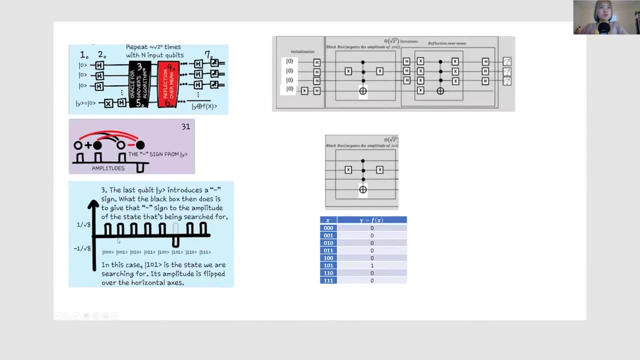 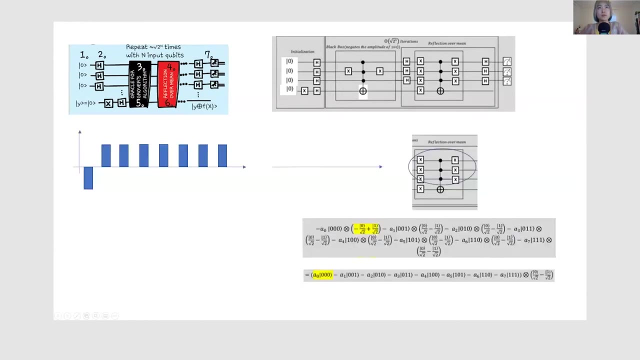 This negative sign will be introduced to no one else except the one that you label. The 101 now gets a negative amplitude. This would be very useful in the next few steps. Look at the second part of the algorithm, this another box. This is like the oracle earlier. 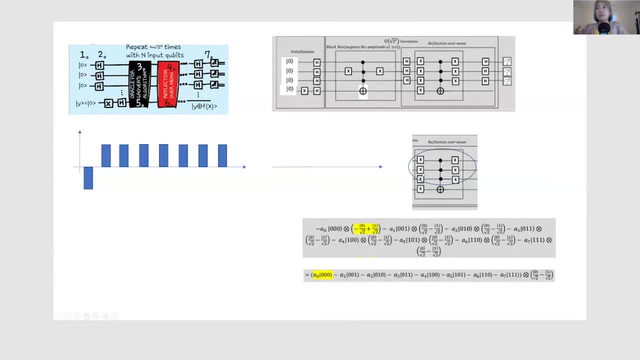 where you have now the x-gates for all three of the input qubits. Because of your experience with the earlier one, you know that if my qubits are all zero, then they are being flipped and then they can control the very last bit. 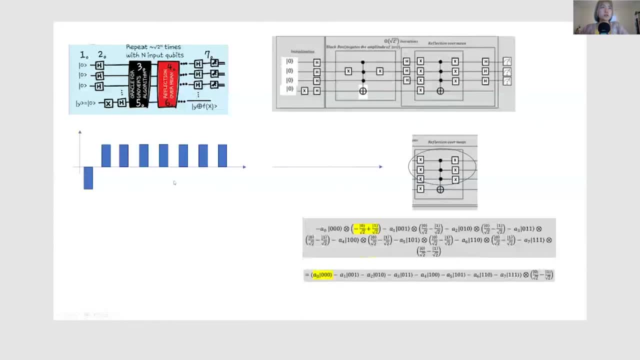 This one allows you to get the 0,0,0 to have a negative, just like how this one got a negative for the 101.. This one would give a negative to your 0,0,0.. But what happens when you have? 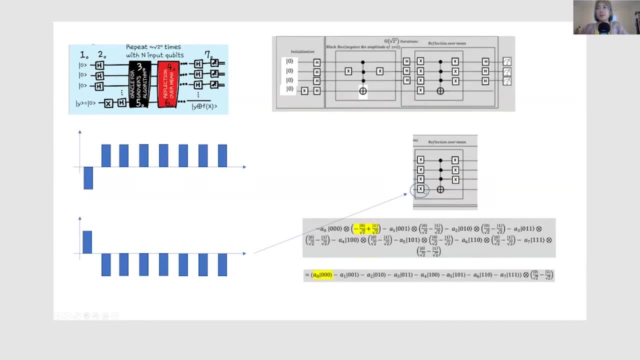 a extra incoming qubit that had a negative sign introduced. What this one does is allowing all of these amplitudes to flip their signs. Now your 0,0,0 becomes positive and all the rest becomes negative. This is the use of this very last qubit here. 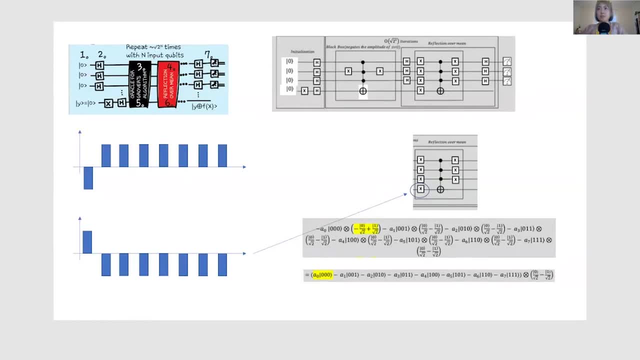 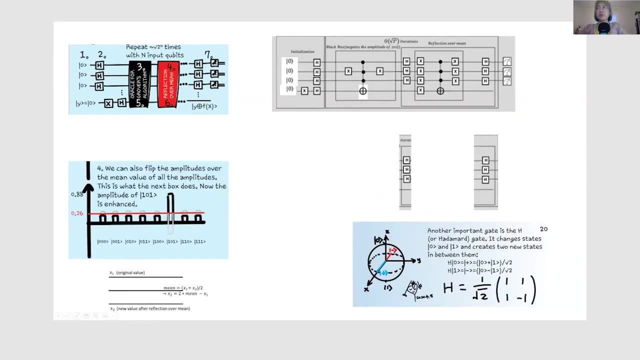 is purposely introducing this negative sign. The next bit is even funnier is that not only do you have this box with all these x-gates, you also have some h-gates on both sides. What does this do This? both sides that you have h-gates? 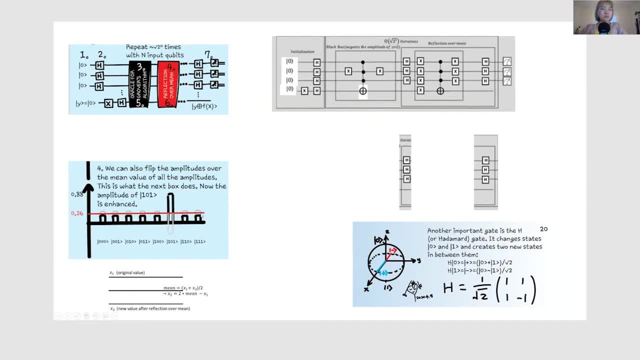 will actually allow you to flip all of the amplitudes over. this mean value of all of the amplitudes. This is maybe a little. if this is the first time you see Gruber's algorithm, maybe a little mind-boggling. 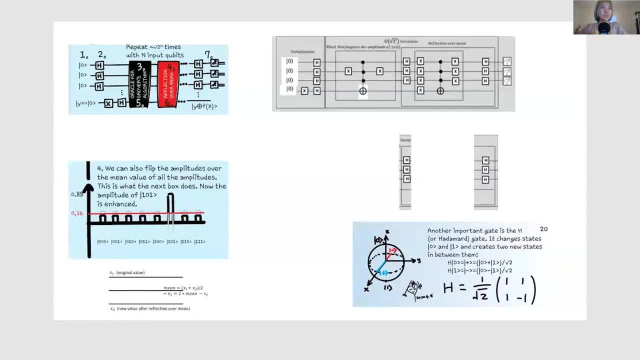 How is it allowing you to flip over the mean, The h-gates? remember that when we look at the single qubit gates, when we introduce h, it is allowing you to go from 0 to plus and 1 to minus. In effect, it is also flipping your states around the mean. 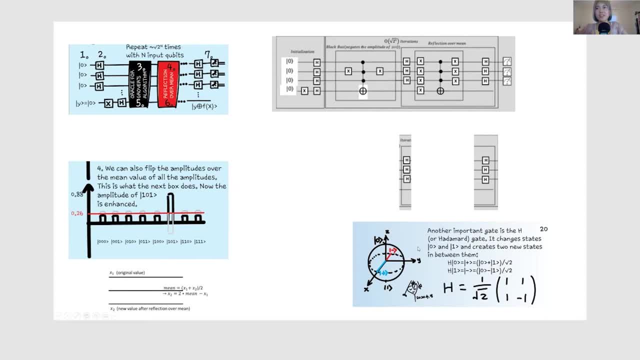 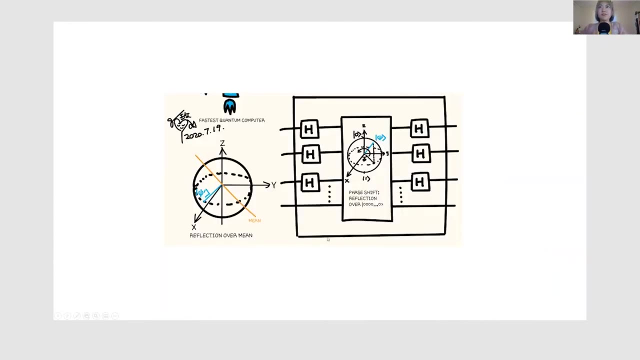 If you have two h-gates around both sides of whatever that's in here. I will show you a little bit more about this. when we do the coding- Actually, I do have this slide here coming up. Let me show this. then Imagine you just have one qubit. 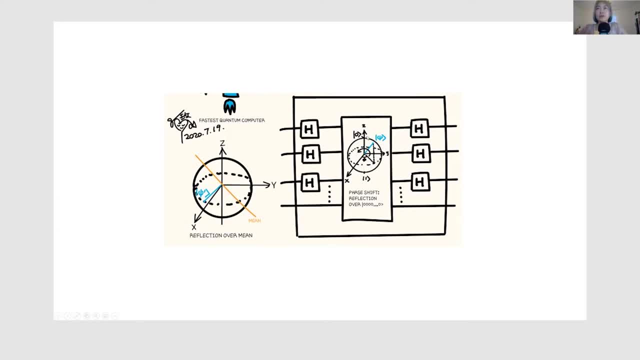 You will just have 0 and 1 as your basis and you have an arbitrary state. We just saw that whatever's in this box is allowing you to have a negative sign introduced, That means you're rotating around this zero axis. That's what this whole box. 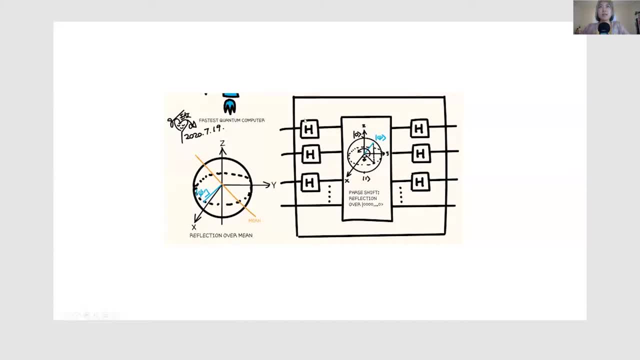 does when you have that negative sign introduced. Now, if you apply this when we have just one qubit, just one h-gates on both sides, eventually your state is going to end up here. That is a flip over its mean value. 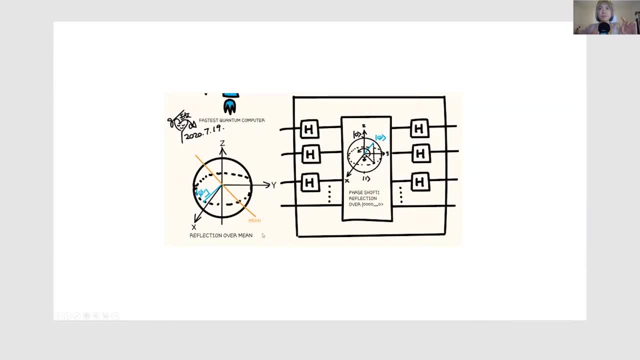 This is just looking at one qubit, So anything that is flipping around the z-axis or flipping around the zero, zero state, plus two h-gates on both sides, will allow you to flip around the mean eventually. So this is only one qubit and we're looking at the Bloch sphere and it's 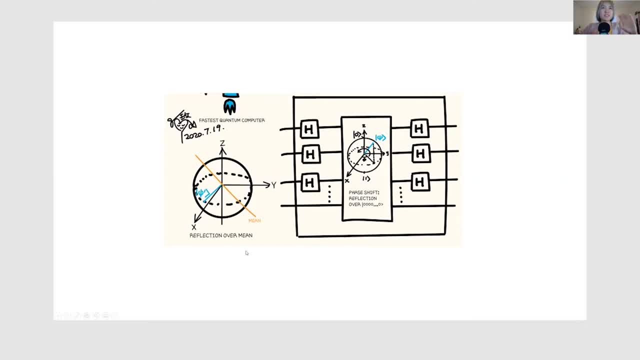 an easy visual tool to think about it. But now, if you have additional qubits, then you're adding up the dimension Humans, we won't be able to visualize more than three dimensions, But the truth is it's just adding more states and it's the same principle. 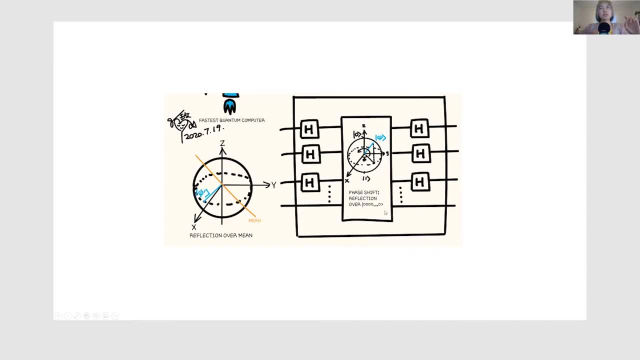 You are flipping over the all zero states in this box and then in this whole box here you're flipping over all of the possibilities mean. So this is really freaky. I really like this, I really like this algorithm. So that's why it is very useful, because now 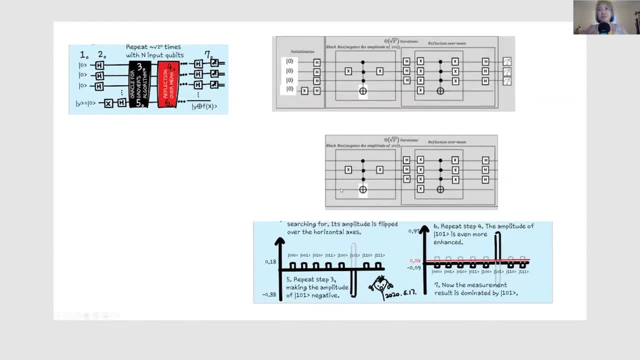 if you repeat this- two boxes over and over- you would be able to continuously increase the amplitude of the first one that you marked. So flip over zero and flip over mean a couple of times, So it turns out that the number of times you need to do 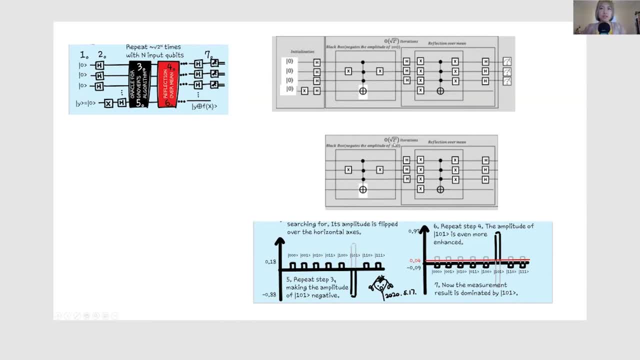 this iteration is square root of two to the n, as I introduced at the beginning of the class. So if you just have three qubits you don't have to iterate so many times. But when you have lots of qubits your classical computer is going to scale with two to the n. 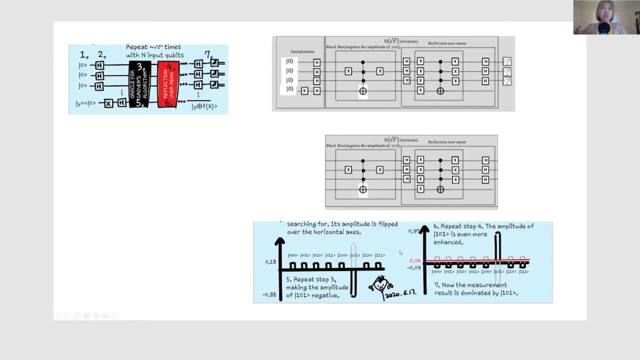 but then Groover can scale to square root of two to the n. much fewer steps Then classical, and that's why it's useful and gives us that speed up. Yeah, Even if you just have a few qubits, you don't also even have to use any computer. 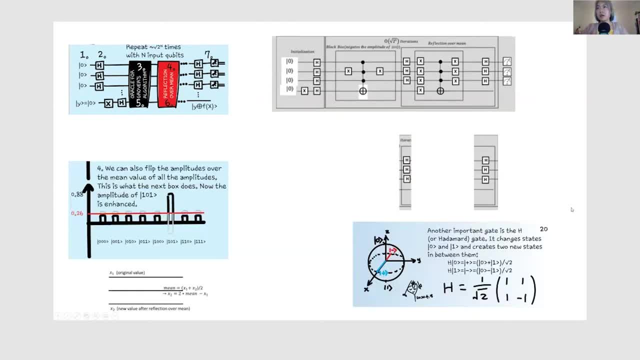 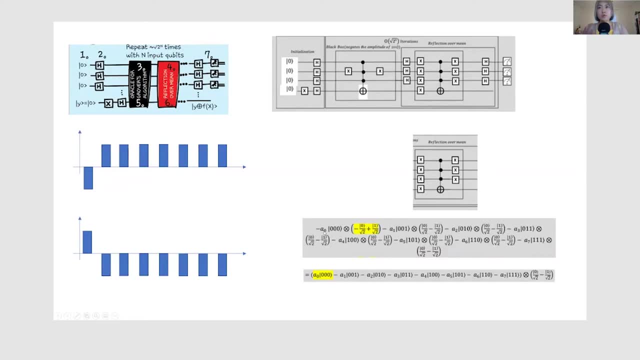 You can just use your brain. I think earlier. I do want to mention that I put the math here. If you want to check what's happening, feel free to just write out. since we only have three qubits, you can write out every single. 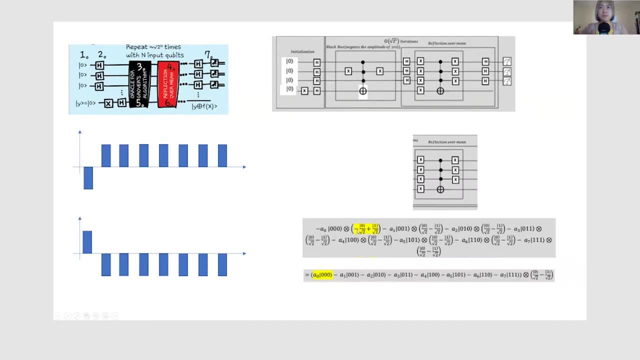 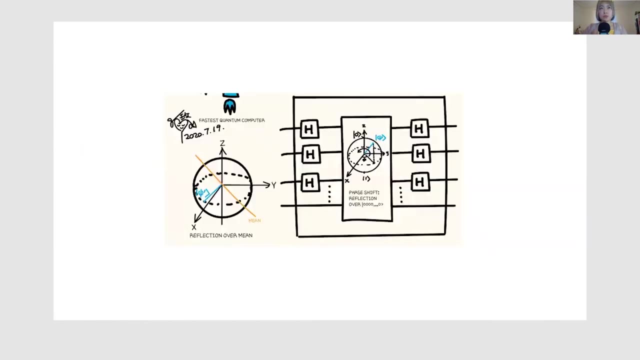 state and see what happens. Then you will see this negative sign will be introduced to all of the possibilities. But then, because your first 0,0,0 already has a minus, it becomes positive. The rest of it will be negative. So definitely try out the math. 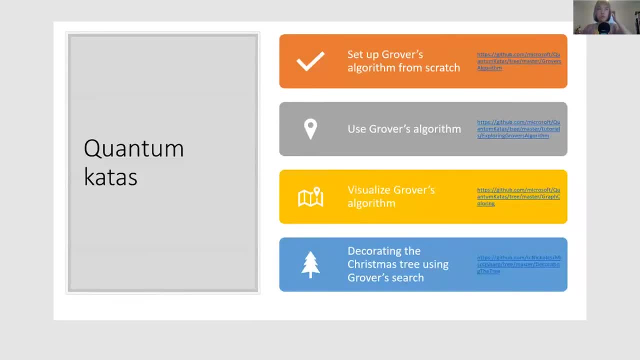 I will highly recommend that. So let's do some coding. We have the quantum cutouts and a lot of samples on Groover's algorithm. What we're going to use today is the one in the cutout, this one, So the one that sets up the Groover's algorithm. 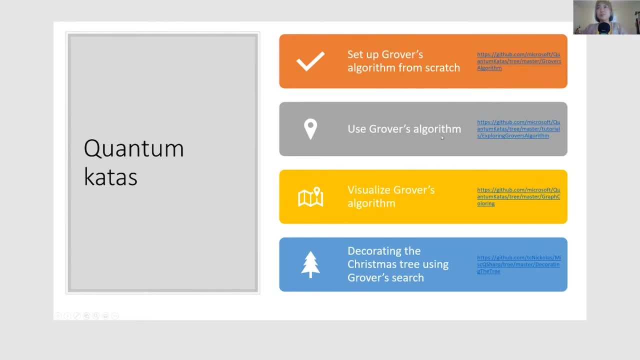 The other ones are using the algorithm, and there are some really fun ones. like this is to use the Groover's algorithm in another setup. This one helps you visualize it by doing a graph coloring example. This one is a fun write-up by my colleagues on decorating Christmas trees. 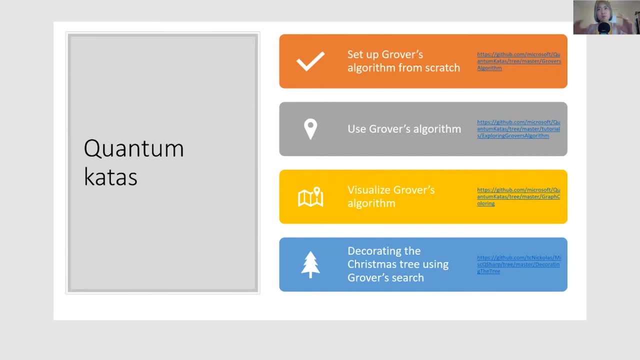 It's like you want to choose. you have a rule of how many ornaments you want to put on each layer of the tree and you need to have efficient algorithm to automatically select where to put what. We also have an analogy by my colleague about Santa Claus trying to find the right. 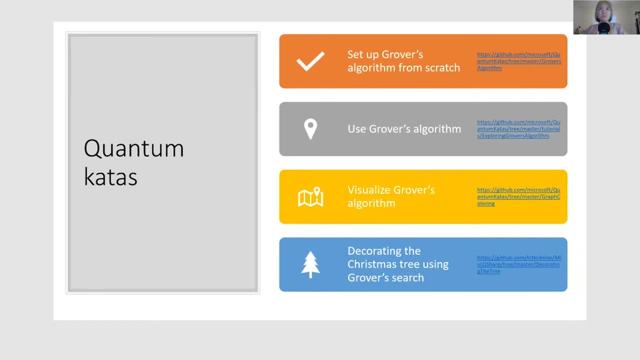 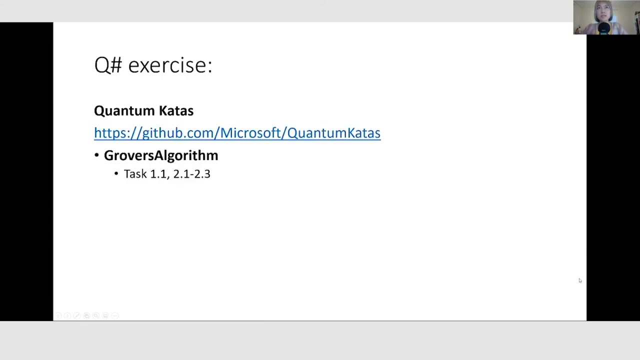 gift for the kids from the bag, but all of the gifts are randomly ordered and he needs to have a algorithm to find the exact right gift. So that's the examples that Groover's can help. So let's go through the cutouts. 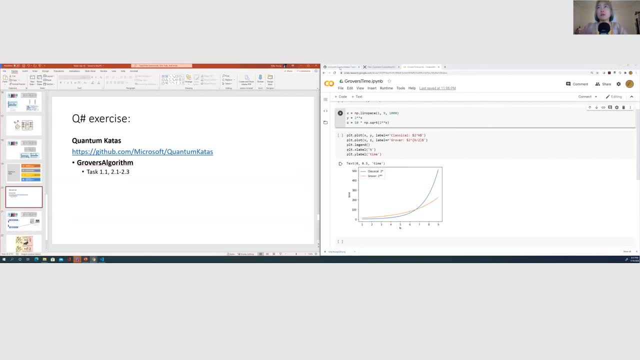 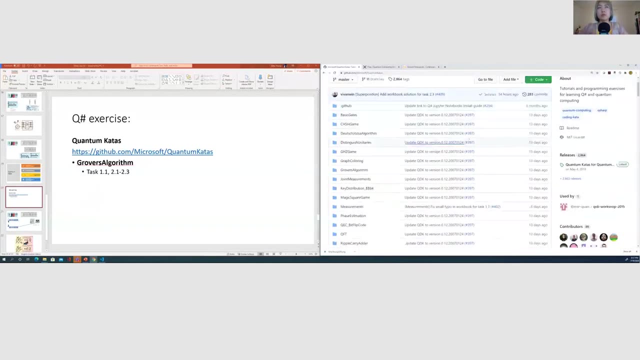 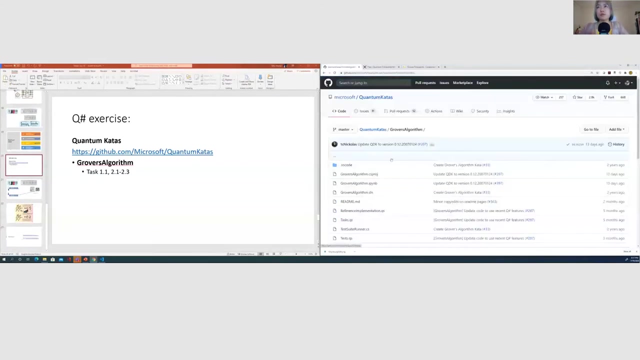 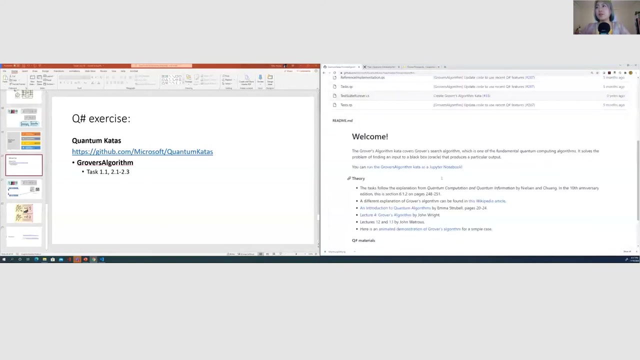 I would show both of my screens. now Do the Control plus to hopefully increase the words for you. You can also do it on your screen. So the Groover's one is this Groover's algorithm folder. Now we will use the Jupyter Notebook. 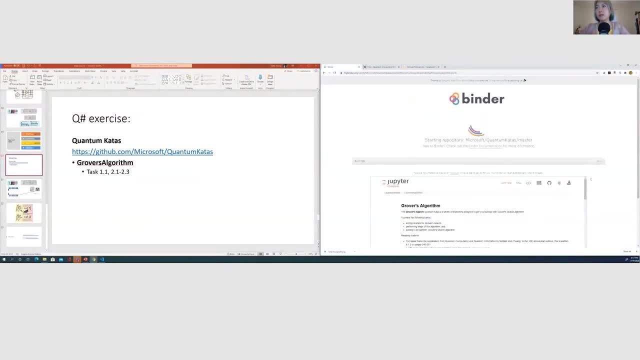 Also, I think we probably can spend a couple classes on Groover's. If we don't get to finish everything, we can continue next time. There are so many interesting, interesting work around that. Hopefully Jupyter is not too slow. 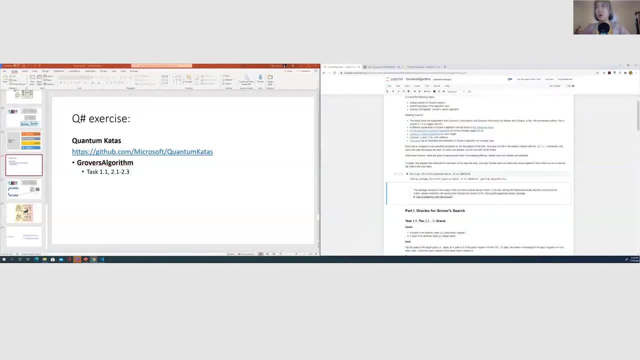 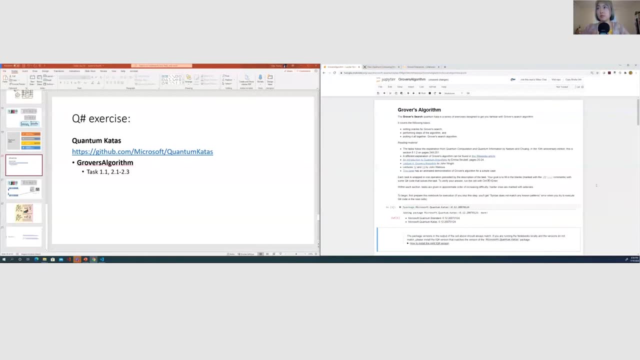 I mean binder is not too slow today. So when you open the Groover's algorithm on the cutouts, this is the non-installation option on Jupyter Notebook. on the binder, Feel free to read the earlier ones when you have time. 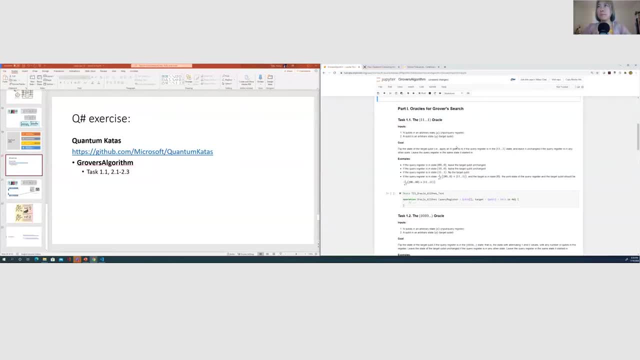 So we're just going to go to task 101. here We are given n qubits, as our arbitrary states. So all of our inputs qubits, So all of the first ones, But in this case we have n, not just three. 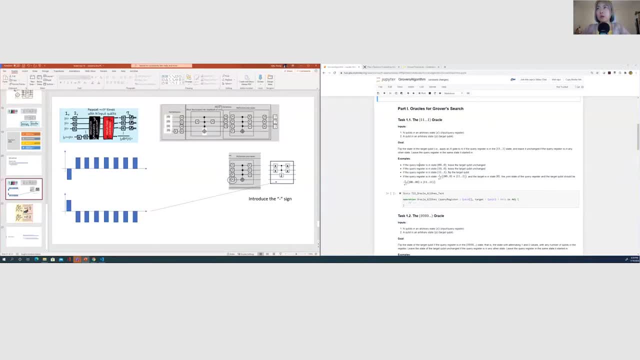 That's also, by the way, why a language like Qsharp is powerful is that we're not limited to a small number. We can scale it up. We can scale it up to any number of qubits. Then we have a arbitrary state y. 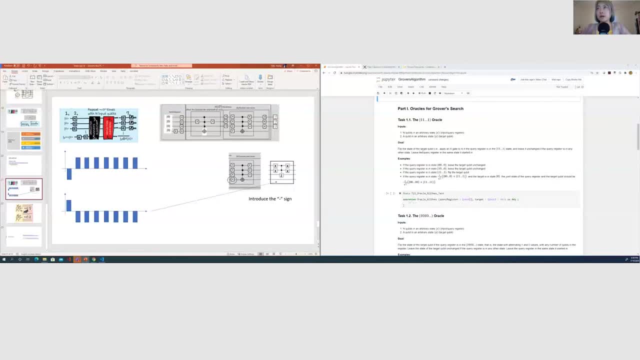 which is our very bottom one. It says: flip the state of the target qubit. apply a x gate to it if the query register is in the all one states. So this is basically saying that we want to label our all one state as the one we are looking for. 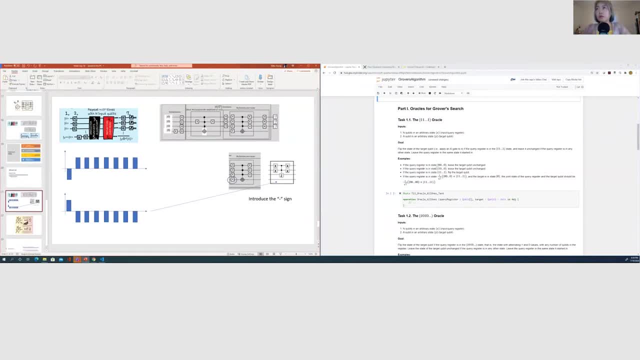 So if the query register is in the state all zero, leave the target unchanged. If it's one plus all zero, leave unchanged. So if you have any zero in your state, leave them unchanged, Only the all ones. you flip the target. 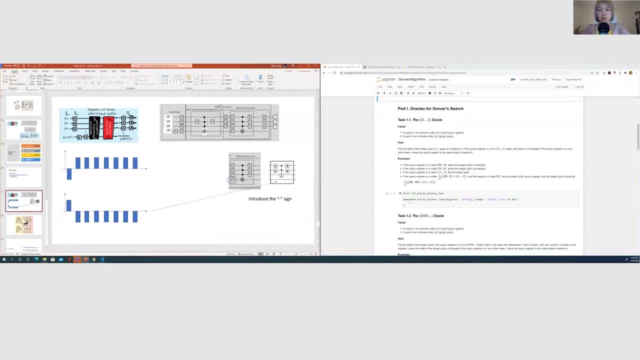 So we just set up what this shows here, And So we just set up what this shows here And don't worry about this, This is for later. So this over here is: yeah, so this oracle, all ones test- is asking us to build exactly this oracle here. 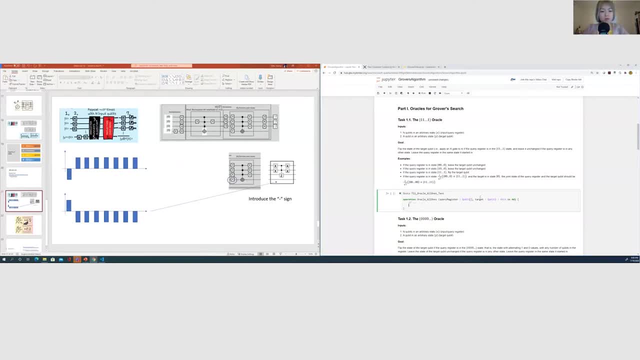 except it's the all ones state that we want to do So. that's actually very, very simple. We use the Control X, exactly like these Control X, And we make all of the query register as our inputs, And then the target is the target. 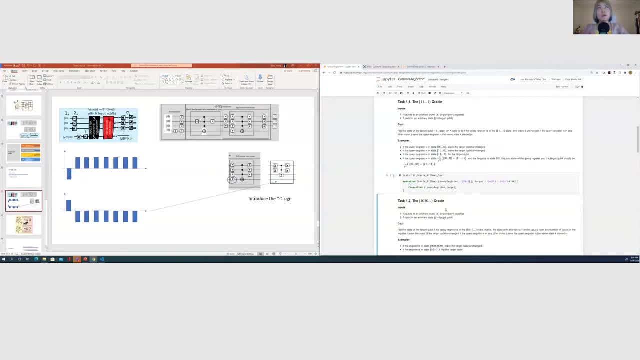 So that's it, Because this one is basically the easiest one. Oh, did I miss anything? Oh, target, This one is the easiest one because you don't have to add any additional X gates. But if you are asked to do like the later ones, 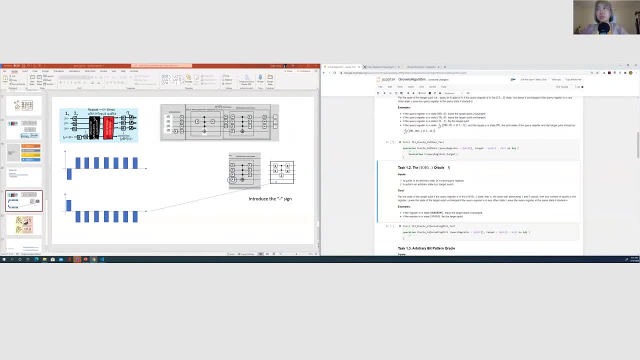 that you actually have to flip the zero states to the one in order to have this control operation working. We're going to skip the next three oracles. Those are for you to do as homework. Those are just setting up different types of oracles. 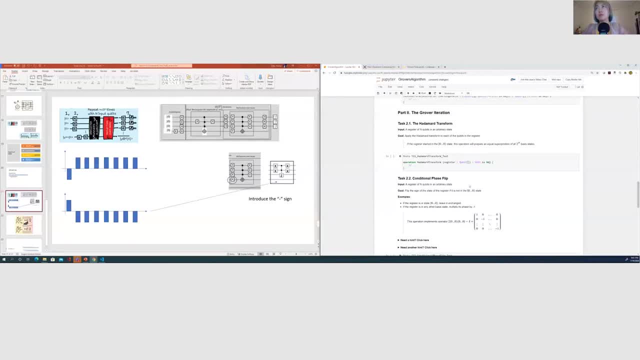 And then we should go build up the Groover iterations. Now is asking to do the Hadamard transformation. So is this part of the algorithm? here is the flip over main. So this is asking to build using the N qubits. 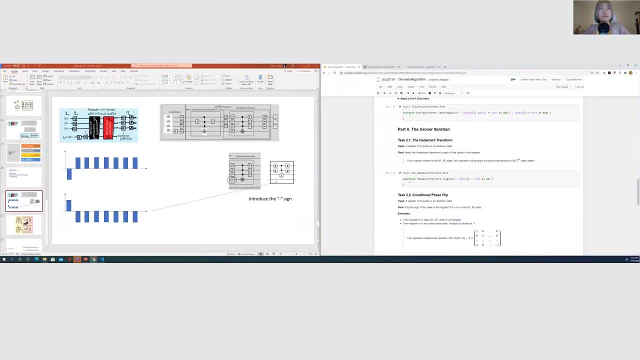 our registry qubits, so all of the top ones, and apply the Hadamard transformation to each of the qubits in the register. If the register started in the all zero state, this operation will prepare an equal superposition of all two to the N basis states. 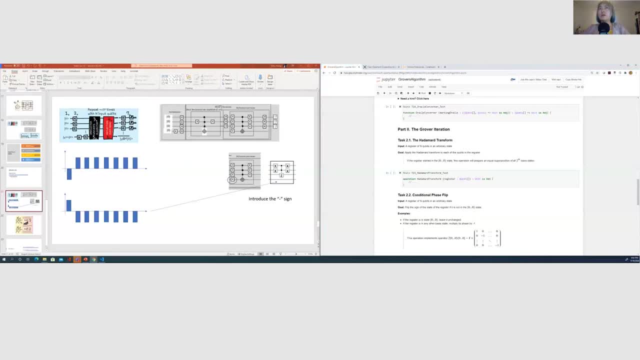 Sure, So yeah, Okay, I was going to talk about this, but now is the next step. So this is nothing but setting up these Hadamard gates, Actually just these, these ones, the inputs. So again, you're going to do the Hadamard. 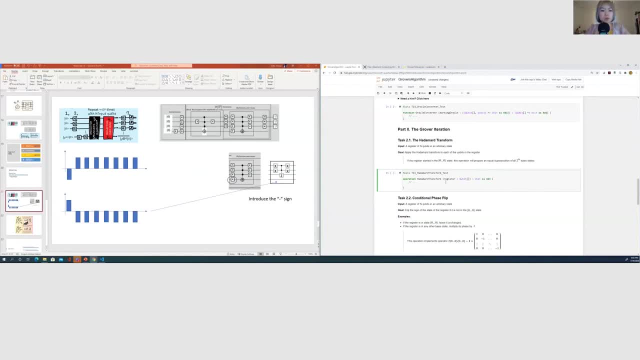 We have a very convenient command called operation, called apply to each, So that reduces your writing. You don't have to do like three lines because you can write like four. all the qubits in your register do at each. But we do have a command called 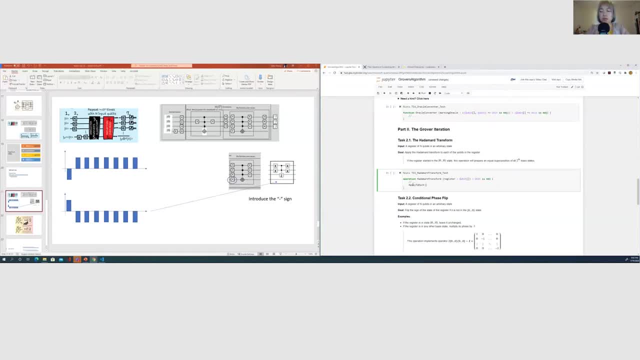 apply to each and you can just do the each gate to register. But here is asking for an adjoin. We have also a very convenient way to do that: You can just put A as adjoin. We also have a control type, So if the question asks us to build control, 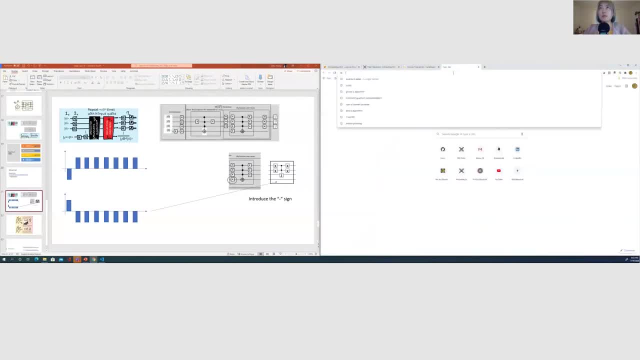 we would put the C there. How do we find it? Let me find out about what these all mean. We can go to the Microsoft Quantum Documentation page. That's where you can find all the APIs about Qsharp. So if I put apply to each, 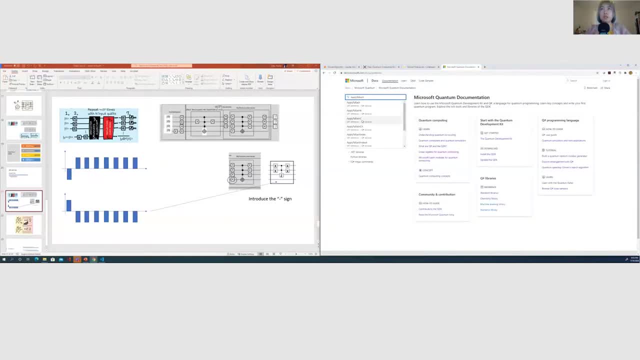 there are apply to each without anything at A, C or A C, So this is the one we're using. You can read about what this operation does. So A here is just the adjoin, and we talked about adjoin some classes ago. 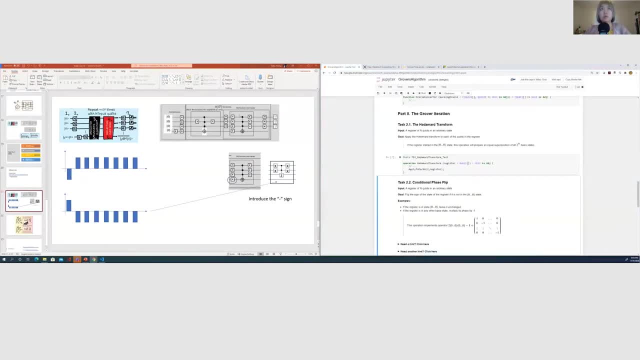 So that's what you need for that step this here. So the next part is fun. I also learn about this part from the Kata's, because earlier I didn't realize this and this, and it's really cool that there are actually many ways you can introduce the minus sign. 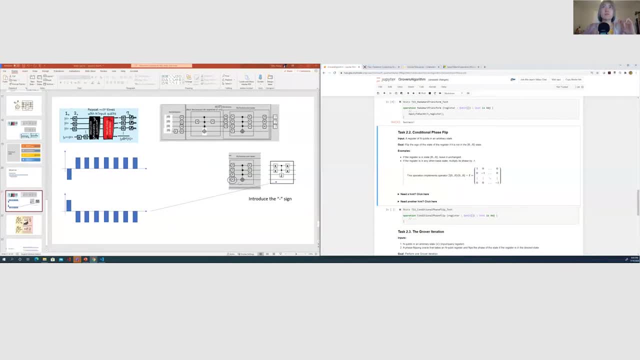 The one that I show you was because it's very similar to this part, So I was naturally showing you this option where you have all of the control ones to. you need to make all of your control ones to be one and the last qubit to be target in order to introduce. 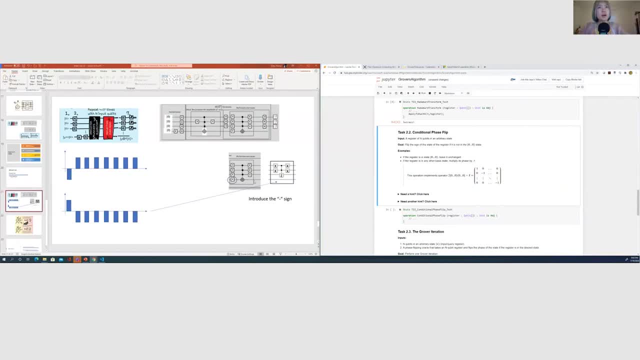 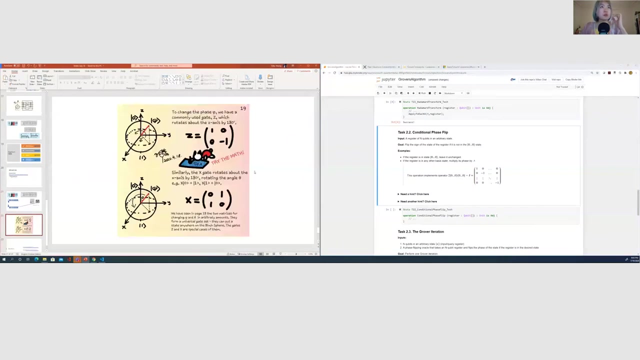 the minus sign from here And then you have to use the minus sign from the last qubit. However, you have other ways to do that. You don't even have to use this very last qubit in this reflection over mean operation, Remembering our single qubit gates. 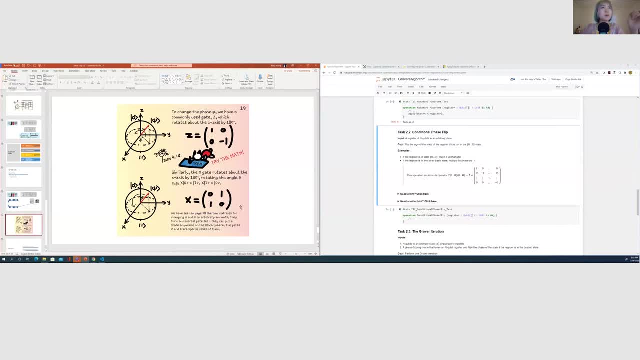 we have seen the x. what x does is flipping from 0 to 1, 1 to 0. But we also have this z gate: The minus sign is rotating around the z-axis. So you're giving your second element, this negative sign, here. 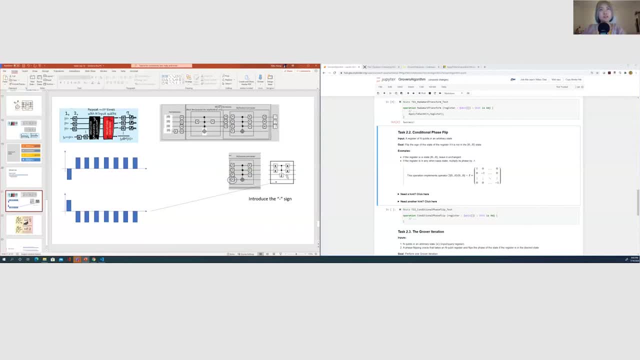 And you can just do this- to introduce that minus sign, And this is what this conditional phase flip is asking us to do. But you can also build this one if you want. So this one is trying to give us a hint to do this kind of. 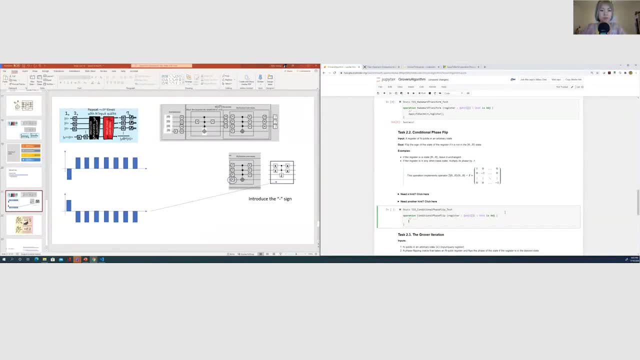 you know a very simple operation, So let's do their way. So the first thing is that you need to set up these x. ah, sorry, use this one now. Set up these x. control the x gates and then the controlled z gate. 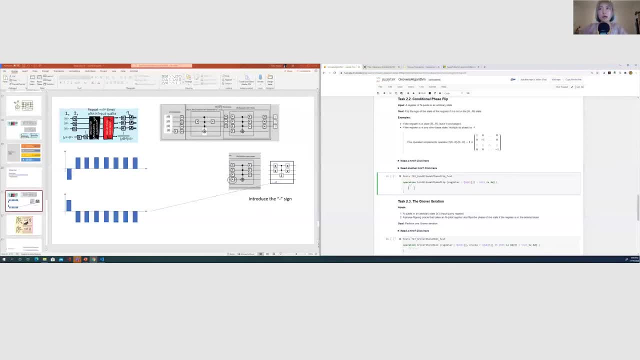 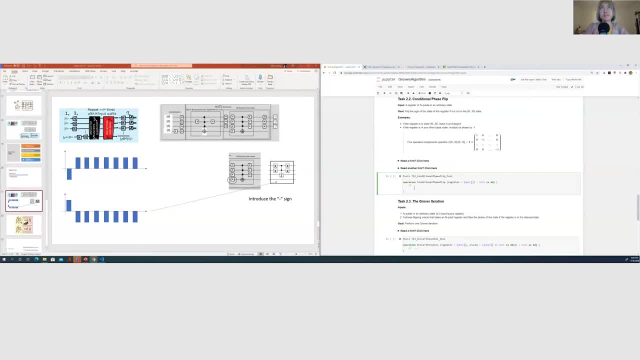 So you can do it introducing quite a few operations. So there's something called within apply. So that means it's exactly like what this is, It's within these things. you can apply this here, So you can do within again, apply to each. 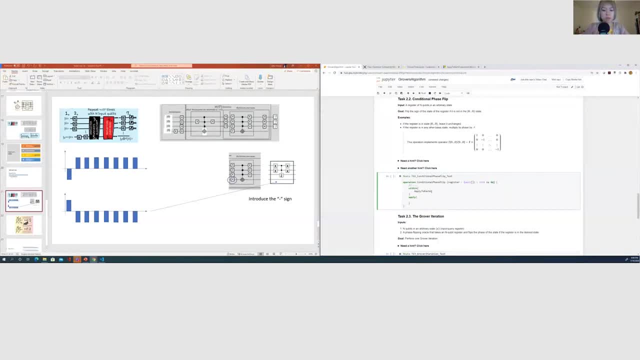 Again it's asking for the adjoined version. so we put an A there, the X to the register. Now in here we are doing the Control-Z. So how do you write in the most efficient way that you want the last qubit to be your target? 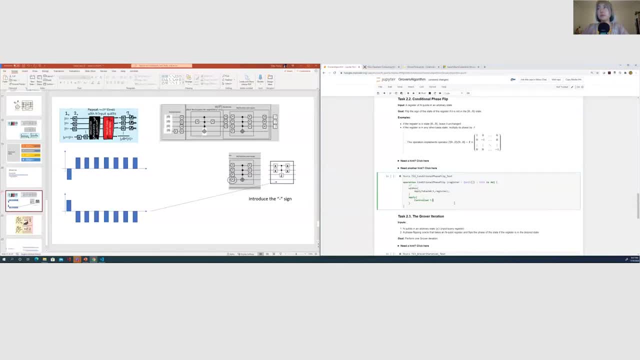 the rest to be your target. The rest of the qubit is going to be controlled. Turn out there's something in Qsharp you can do that, and that one is called the tail. If you look at the API, the tail function returns the last element of the array. 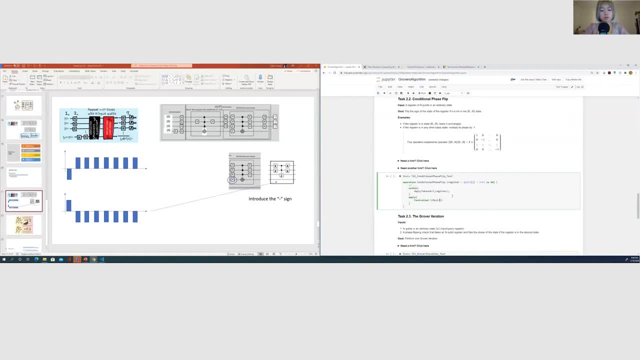 Opposite to tail is most, So most is all the rest of the qubits and tail I think I might have left out. I think we need to have the X for these ones too, So that's what this is helping us to set up. 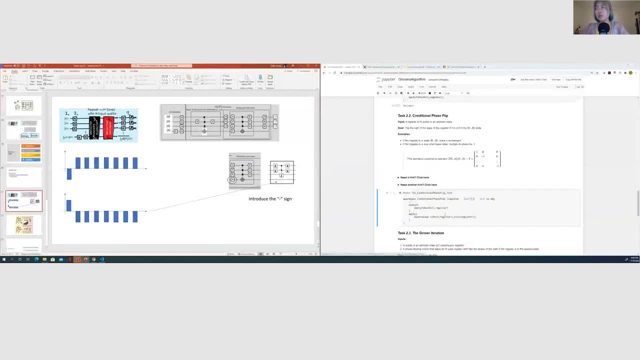 So that's how you can do a conditional flip. All this does is introducing to you. I might have left some brackets. Good point. So I'm using this operation without opening the right package at the names database, So you actually have to open it here in order to use. 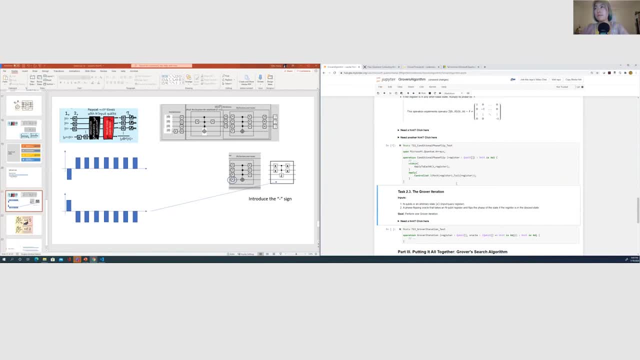 the library. So that should do it. The very last step is allowing us to put everything together, So doing the iterations. So it's exactly like what we set up on the left here You just do because Oracle here is already introduced. 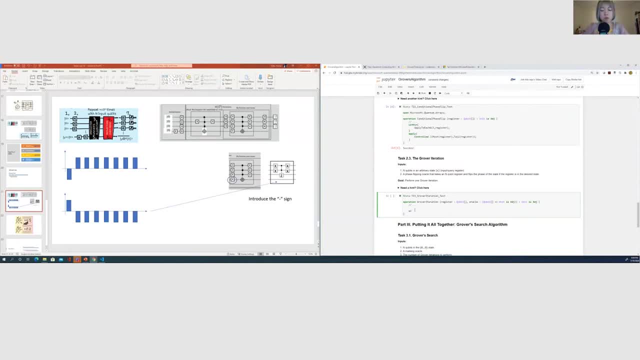 and this is your Oracle. You write Oracle register and then you have the Hadamard and we had the Hadamard transformation defined here, And then this was the, for the Last step is the rest of the Hadamard gates. let me do this again. that should do. 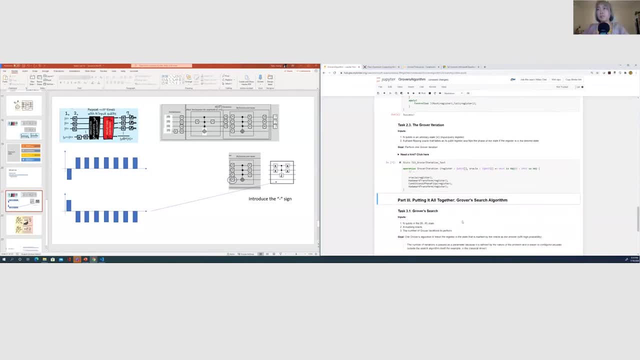 This is how we set up step-by-step. See that oracle here. if you just have any oracle setup, then you can interchangeably put any oracle that you want in this step. Also, we have no limitation of the number of qubits and it can be any number. 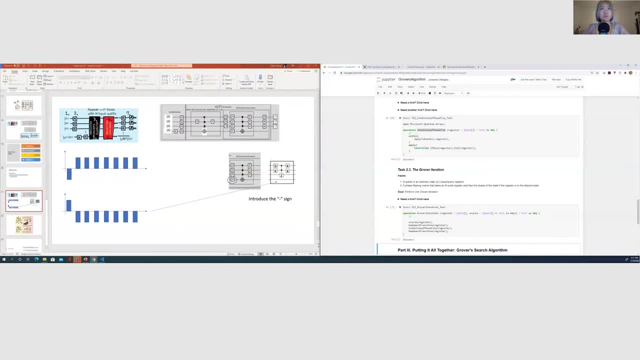 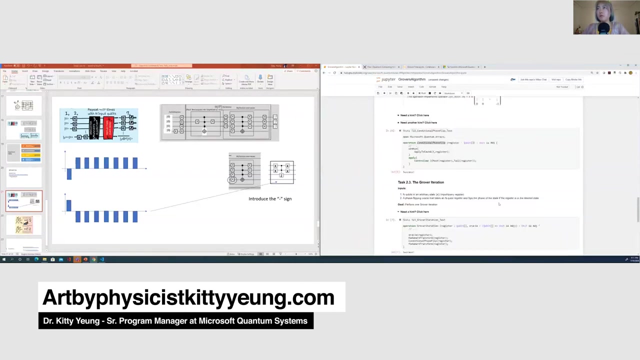 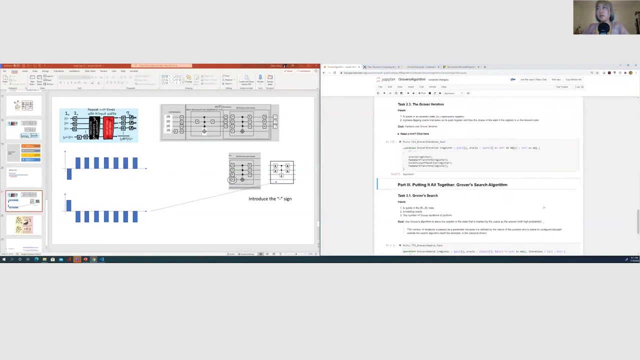 This is just a visual guide for a small number of qubits. We can draw a diagram, but when we want to scale it, it really needs this high-level language for us to represent a scalable algorithm. I will let you finish the ones that we skip and the last bit. 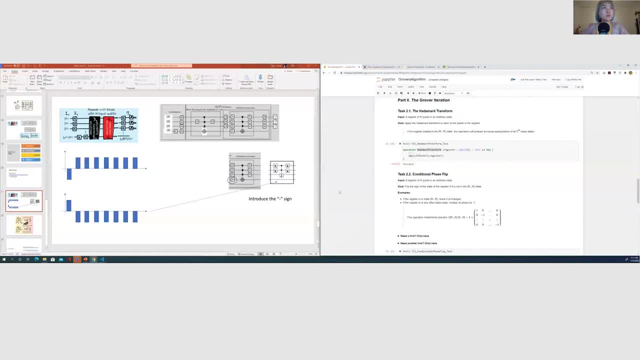 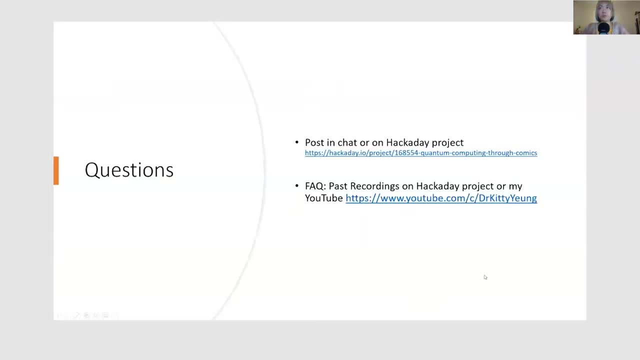 Next class. we should probably try something else around. Groover Frequently asked question. all of the recording is posted on Hackaday, on the project and also on YouTube. I have a few minutes I can look at in the chat if there's any question.